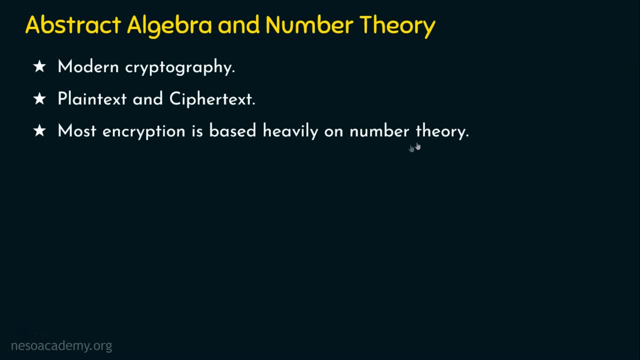 are heavily depending on the number theory concepts. Not only number theory but also the abstract algebra concepts. So, we are sure that the modern cryptography and the encryption algorithms that are widely used in today's world are heavily depending on the number theory and the abstract algebra concepts. And when we talk about the modern cryptography, there is no major contribution of calculus and trigonometry with the modern cryptographic areas. Anyway, our intention is focusing more on the number theory and the abstract algebra concepts because almost all encryption algorithms are heavily depending on the number theory and the abstract algebra concepts. 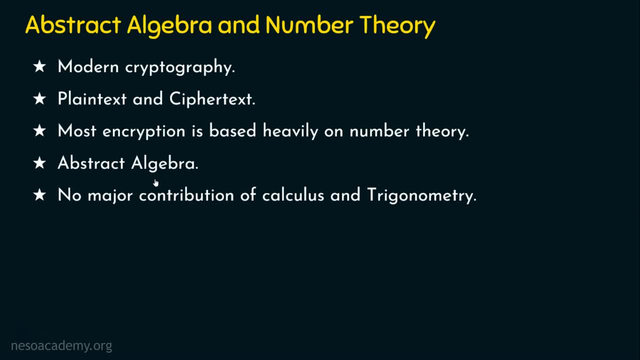 Let's see what are the concepts that are really required and what are all the topics we are going to deal in this chapter. 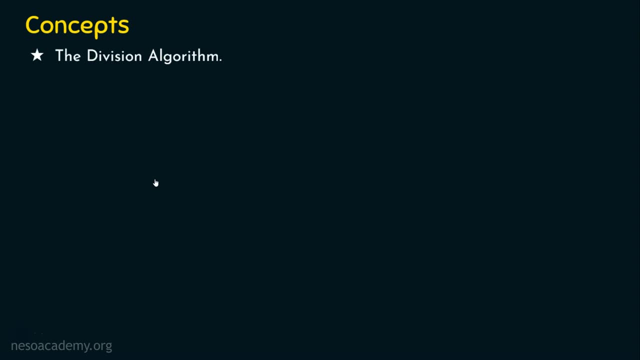 The first concept is the division algorithm. We know in a division algorithm, we get normally two results. One is the quotient and the other one is the remainder. Since division algorithm is a basic algorithm, I am not going to touch upon this division algorithm in this presentation or in this lecture series. But still, we should know how to generate the quotient and the remainder. 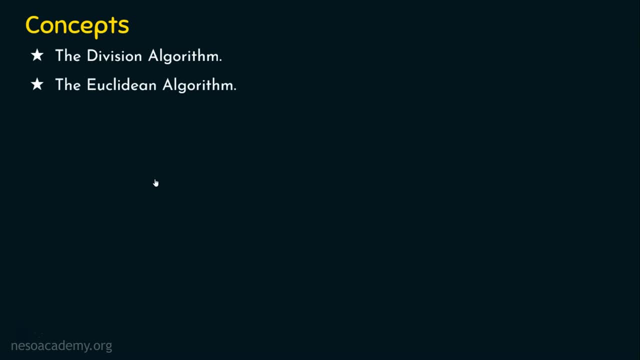 Then comes the Euclidean algorithm for finding the greatest common divisor. So, Euclidean algorithm is a common divisor. Then comes the extended Euclidean algorithm to find the multiplicative inverse. In order to find the multiplicative inverse of a number and that too under mod, we can apply extended Euclidean algorithm to find whether there exists a multiplicative inverse or what is the multiplicative inverse. Then comes the modular arithmetic. Modular arithmetic is very 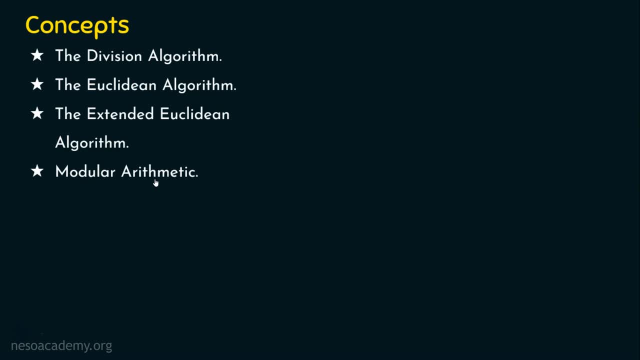 important as far as the modern cryptography is concerned. Don't worry about this now. Anyway, I will talk about the modular arithmetic concepts in the coming presentation. 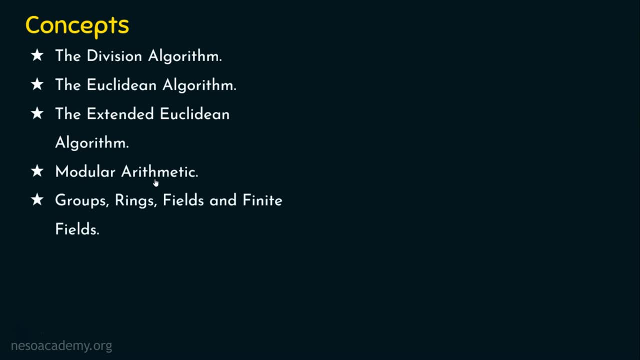 Then comes the important mathematical concepts, the groups, rings, fields and finite fields. Anyway, in the coming lectures, you will understand why groups, rings, fields and finite fields are 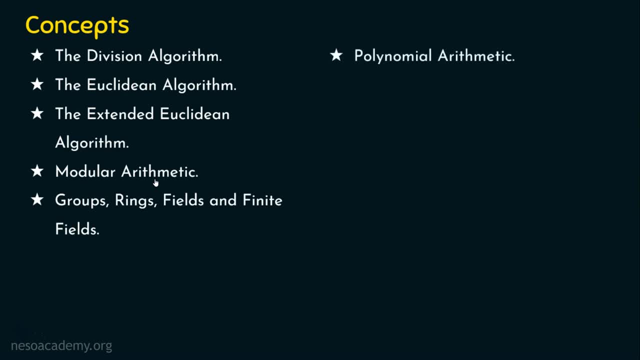 very much essential for cryptography. Then the polynomial arithmetic. Already, we have seen about modular arithmetic which is highly required for modern cryptography. Also, we need the assistance of polynomial arithmetic for better security. Then prime numbers. In cryptography, prime numbers are inevitable numbers. The most widely used algorithms such as the RSA algorithm, elliptic curve 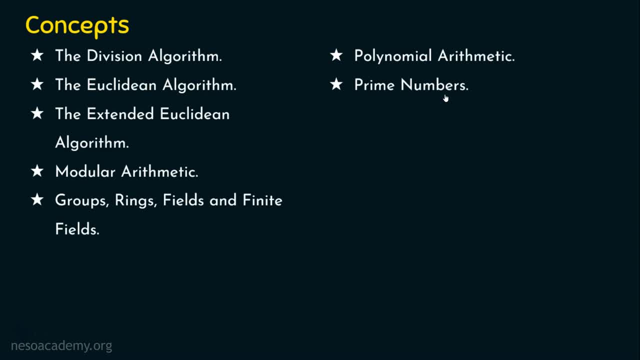 cryptography, Diffie-Hellman keys, all these are truly depending on prime numbers. Then the Fermat's and Euler's theorem. I'll explain about these theorems in the coming lecture. Then comes the testing for primality. I already told you that prime numbers are the inevitable numbers in the modern cryptography because most widely used algorithms prefer prime numbers. But these are the prime numbers. These prime numbers will not be small prime numbers like 5, 7 or 11. Encryption 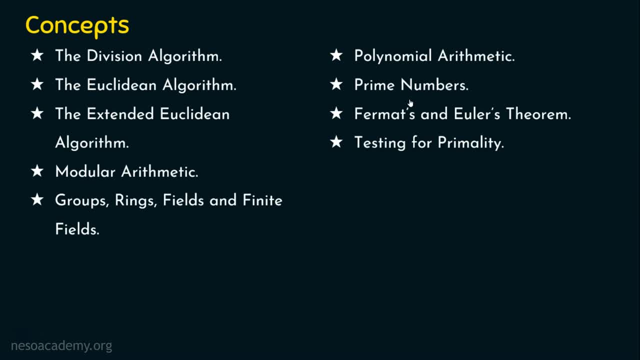 algorithm should take prime numbers which is of large number of bits, right? So, more number of digits will be there, maybe 100 digit prime number or a 200 digit prime number. How to test that number is a prime number? We can't go and manually work on it. So, there should be some algorithms to test whether that number is a prime number or not a prime number. So, we'll be focusing on the 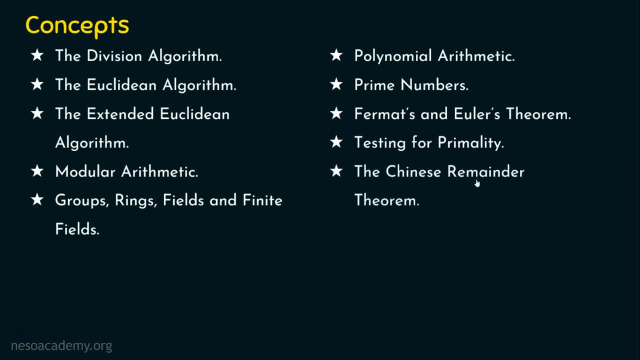 testing for primality and then we have the Chinese reminder. Then finally, we'll be focusing on the discrete logarithms. The topics what I have mentioned is just limited topics. Cryptography deals with a lot of stuff wherein we are going to focus almost on 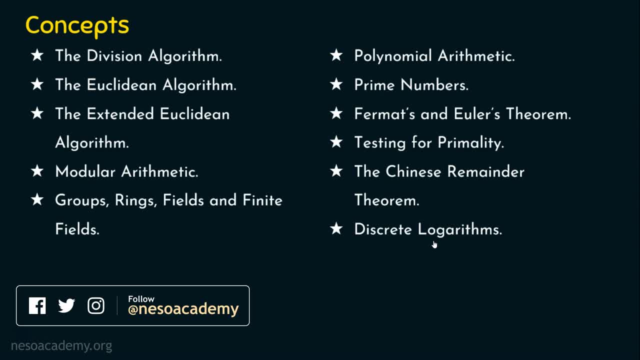 all aspects. But still, we need to know that mathematics plays a major role in dealing with the cryptographic areas because this number theory and abstract algebra are very much important for cryptography. Before we conclude, let's see about the few interesting things about 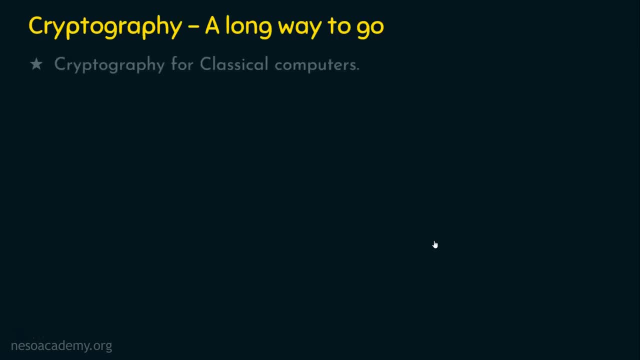 cryptography. It's not a simple way. It's a long way to go. The current computing system will become classical computing when quantum computer is successful. So, whatever computers we have, whatever computing system we have, all these will be referred as classical computing if quantum computer research is successful and quantum computing is achieved. What's so special with quantum computing? Because this quantum computing requires less power when compared to classical computing. Also, quantum computing is a very important part of quantum computing. So, it can execute, I mean the quantum computers can execute tasks faster and more accurate than 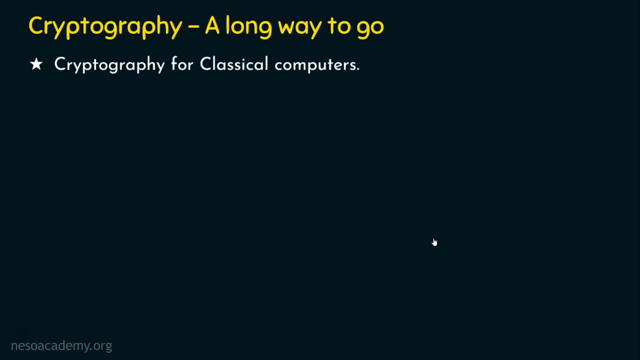 classical computing. In the traditional computing, that is in the classical computing, the atom changes very faster. Whereas, in quantum computing, the atom changes even very faster than classical